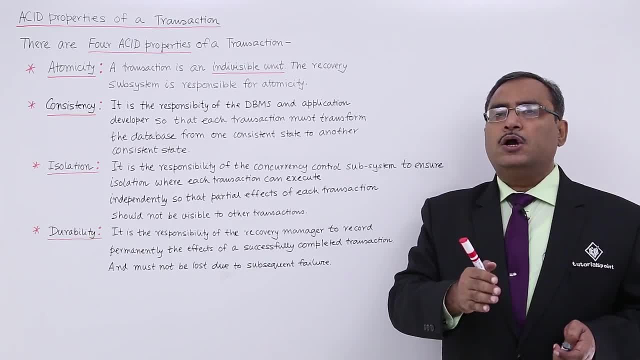 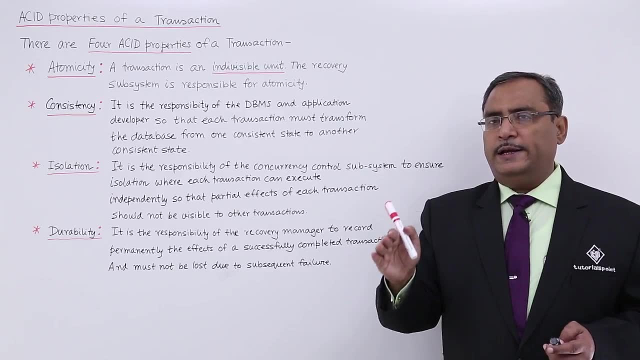 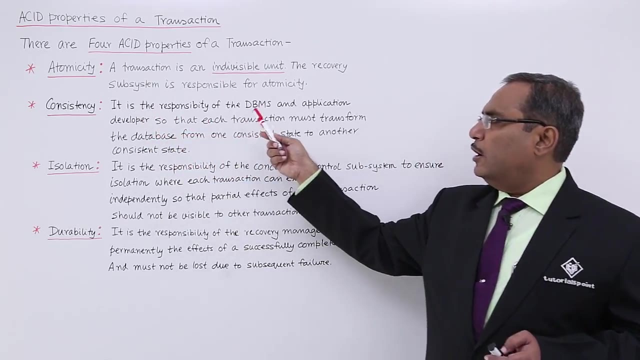 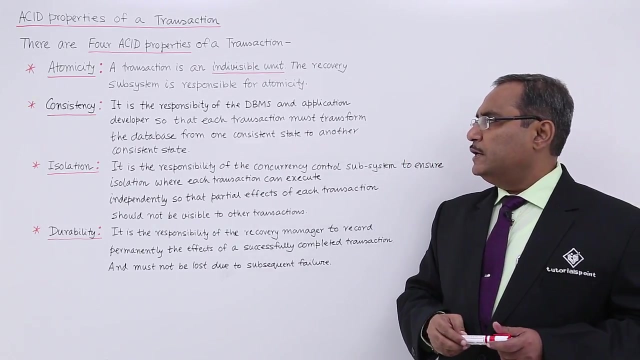 executed. before that, the database state should be consistent and after execution of the transaction completely, the database should find itself in another consistent state. it is responsible- it is it is the responsibility of the dbms and application developers so that each transaction must transform the database from one consistent state to another consistent state. so, prior, 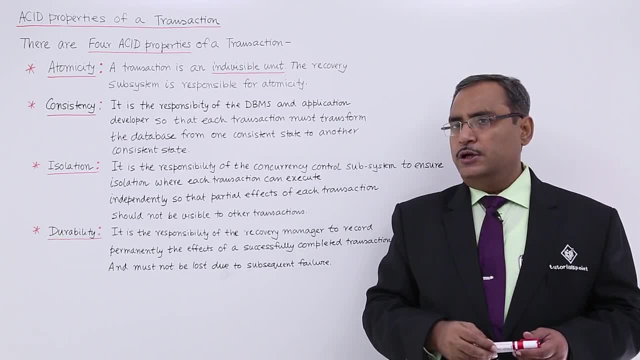 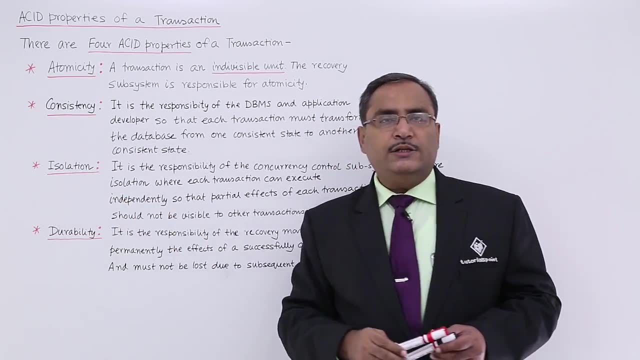 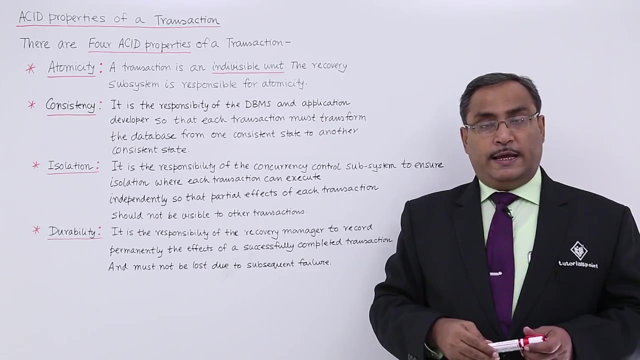 execution of the transaction and, after execution of the transaction, two states, whatever the database is having, must be consistent. ok, next one is our isolation. we know that in parallel, concurrently, so many transactions will be executed and taking place. each and every transaction will leave its own individual effect onto. 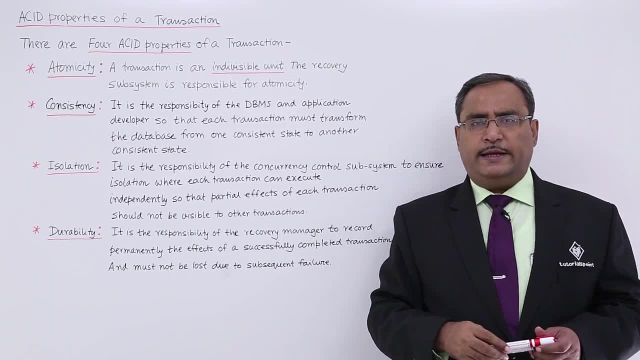 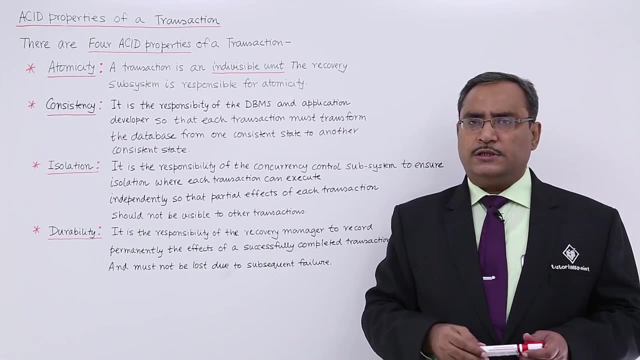 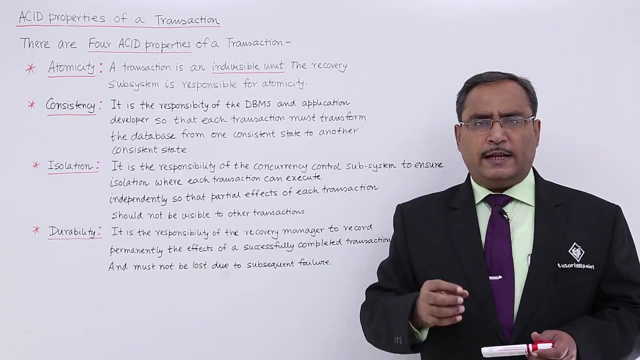 the database. so whenever multiple transactions are taking place at the same time, say in case of credit card server, so server which is dealing with credit card related transactions, so so many card punches are taking place, swapping are taking place, so so many transactions are reaching at the same time, at the same instant of time, concurrently, in parallel to the database. 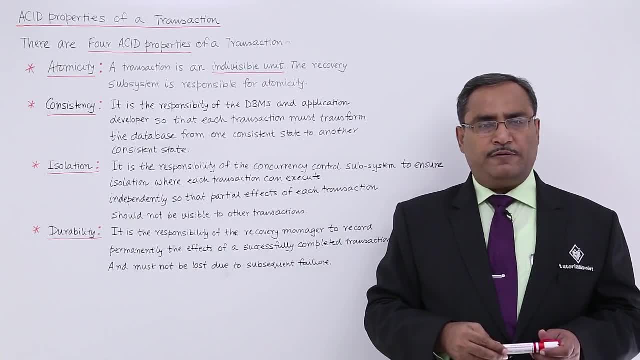 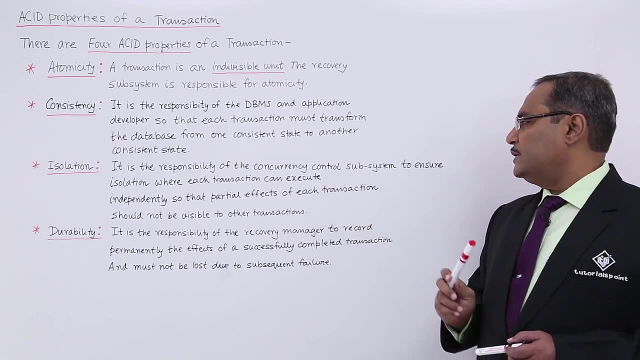 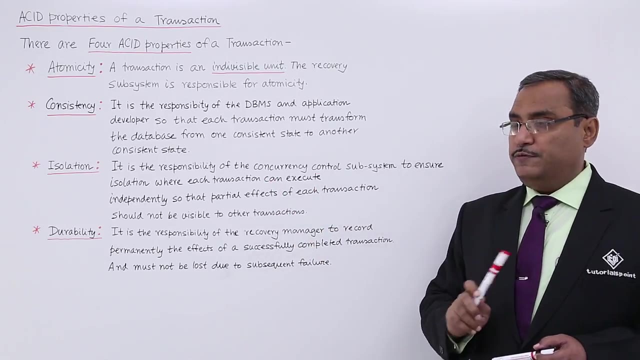 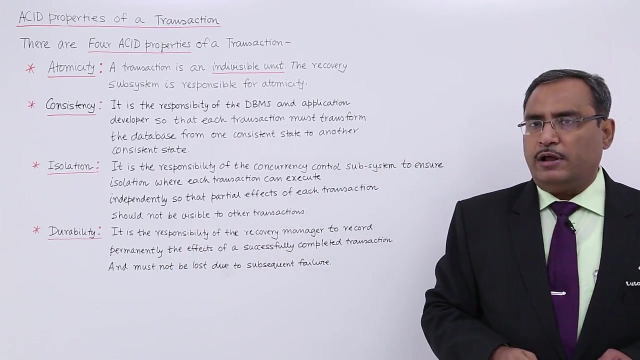 server. So these transactions will leave their individual effects onto the database. so it is the. it is the responsibility of the concurrency control subsystem to ensure isolation, where each transaction can execute independently. so that is very important, so that partial effects of each transaction should not be visible to the other transaction. so that is why each and every 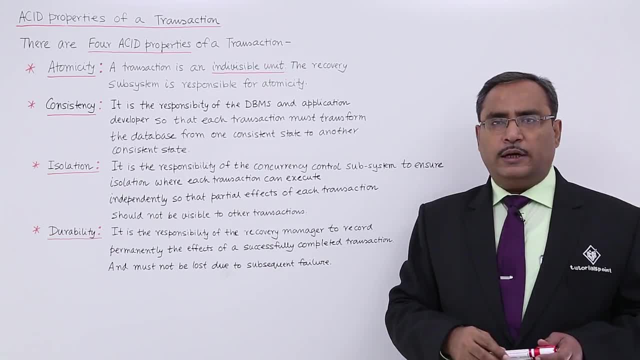 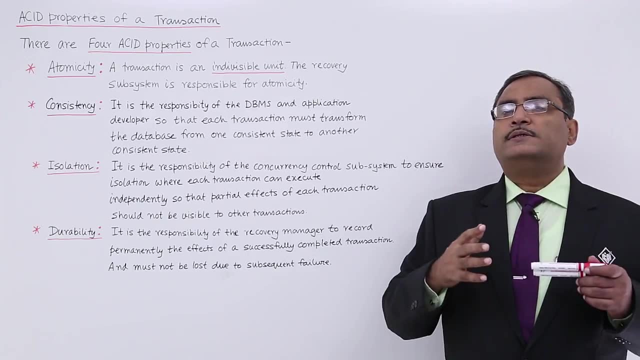 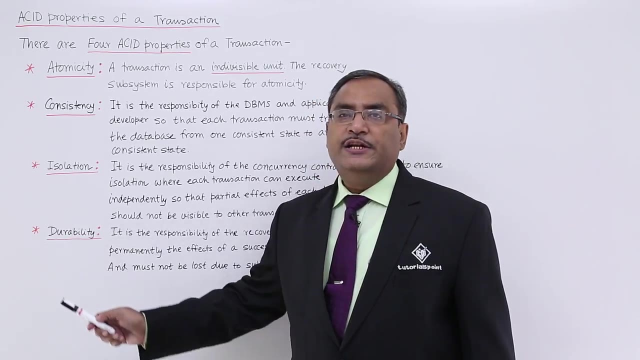 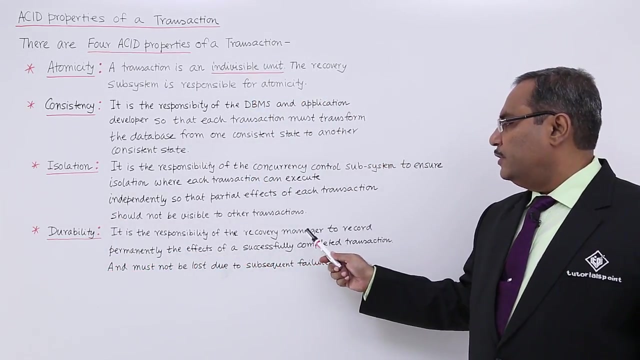 transaction will leave their individual effects onto the database As if that transaction was working in solo, not in parallel, not in simultaneously with other transactions. the last property in the ACID property set is durability. here the last letter is D. so that is the durability. it is the responsibility of the recovery manager. 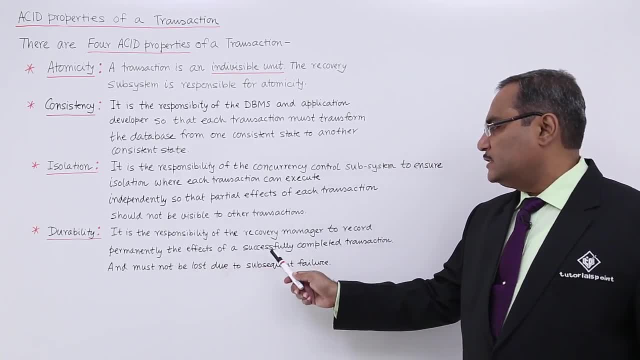 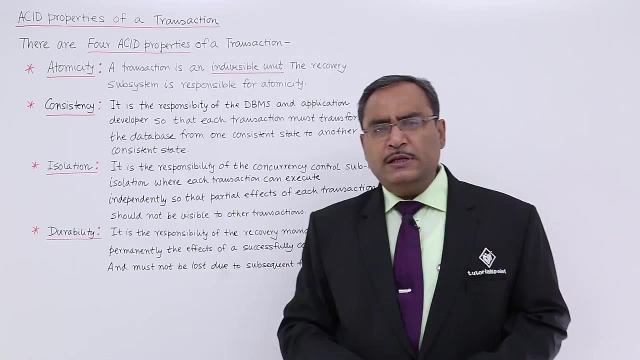 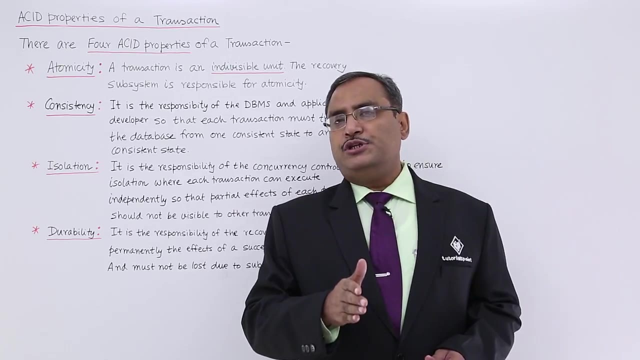 to record permanently the effects of a successfully completed transaction and must not be lost due to subsequent transactions. So that means whatever the transactions are taking place which is making or which is which will have a transition from a consistent state of the database to another consistent state,